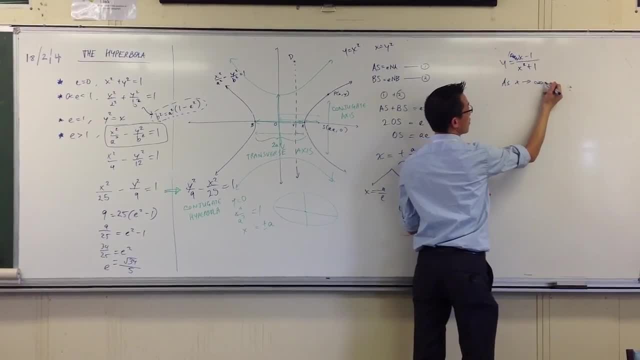 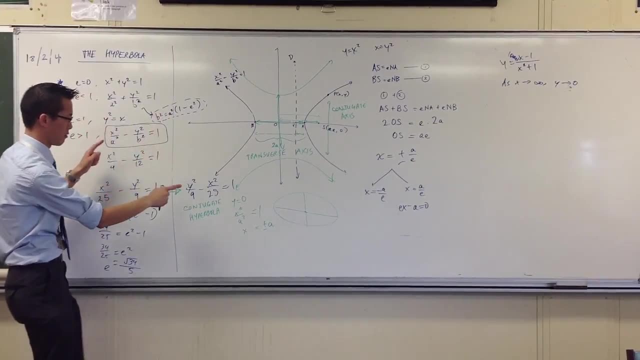 So, as x approaches infinity, y approaches infinity, So it's zero, so it's a five. okay, Now, in order to work out, therefore, what's happening in this scenario, I need to get it in a form where I can say: y is equal to something. 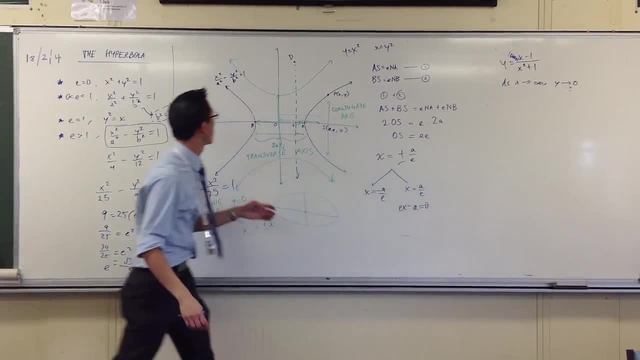 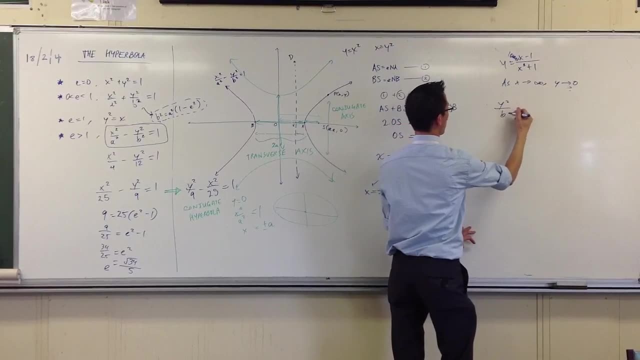 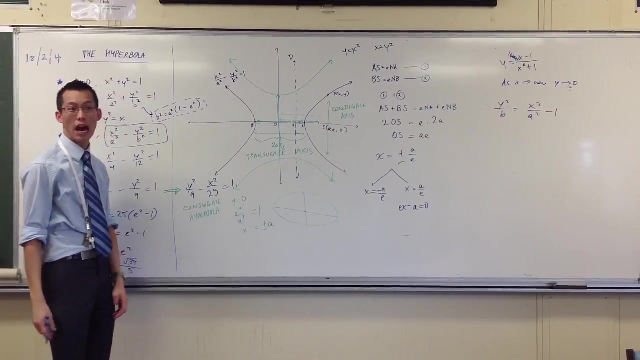 so then I can see how it's behaving. So this is kind of not a very useful form to put it in, so let's make y the subject. What have I got here? y squared 1b, Is that okay? I've just switched it. 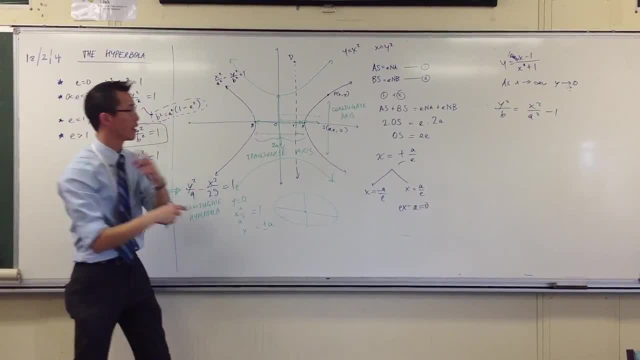 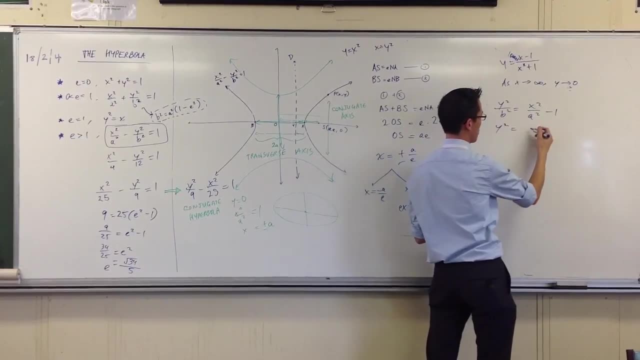 I've switched around the y squared on b squared and the 1.. So now I guess I would divide. Sorry, that's a b squared. I would divide through by b squared, So that gives me 1 on b squared times, all of that. 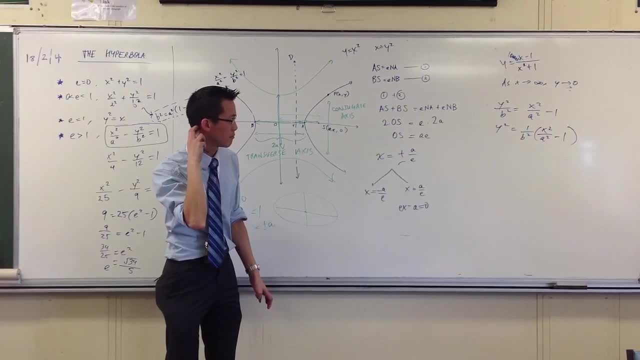 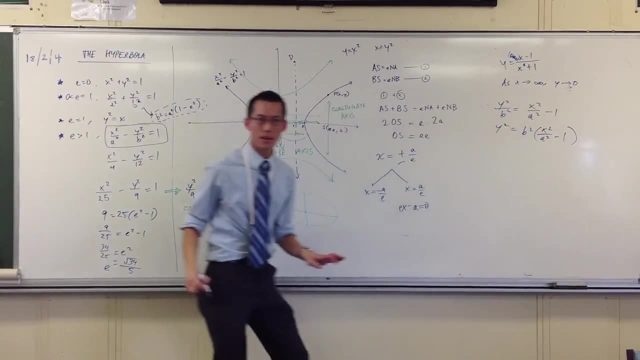 Okay, And Hold on. what have I done? Sorry, what have I done? I should multiply. That's what I should do. Okay, Now, what do I do? I should take the square root, shouldn't I So? 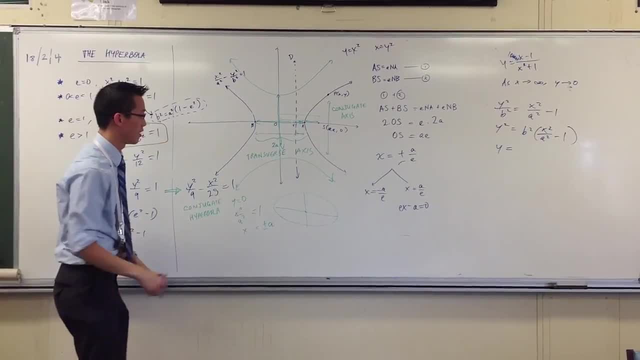 Now, by the way, you're going to get plus or minus, but do you see what that signifies? Because you've got two: Here's the plus and here's the minus, So no big deal. I'm going to be naughty. 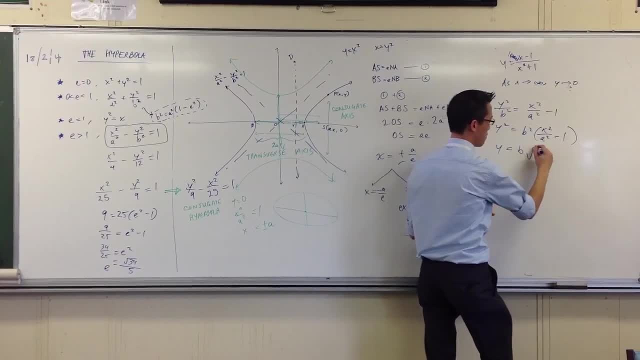 I'm just going to write down one of them. okay, Don't kill me. So I've got the b and the x squared on, x squared minus 1. And we'll consider this case and then just slap a minus sign on it for the other one. 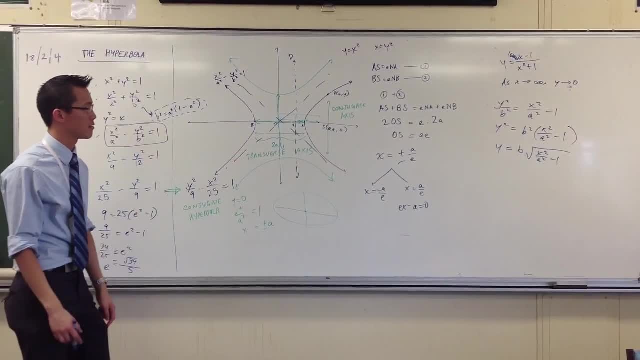 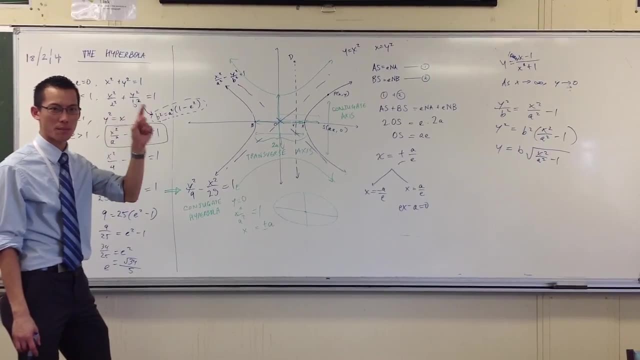 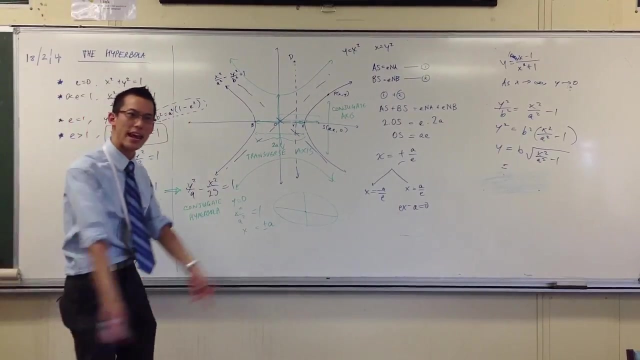 Okay. Now this is okay. This is okay, But I can do a little better than this, right? I'm trying to work out what happens as x approaches infinity. Aren't I What's going to happen? Because, at the moment, as I consider x to infinity, 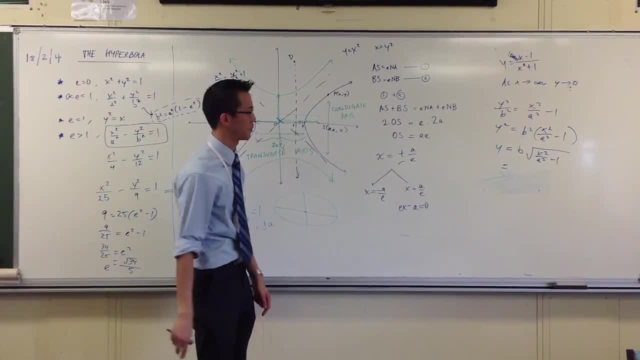 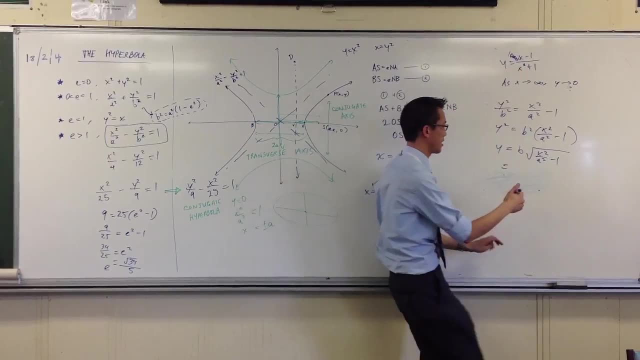 it's not a useful result to me. This is what I was thinking. So limits are useful when you've got things that vanish off to infinity or zero, Right? So that's why I take out this guy. Okay, Watch what happens, right?